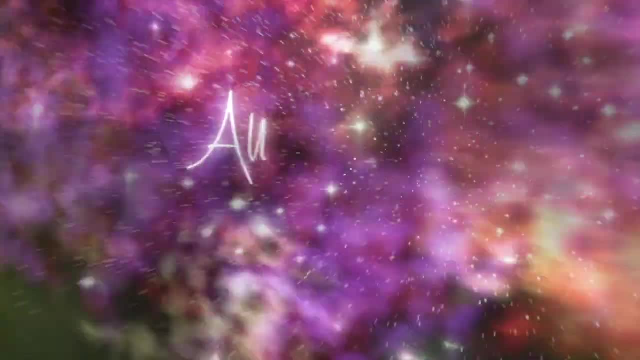 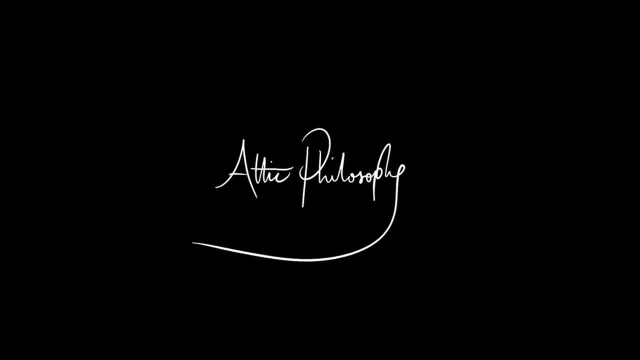 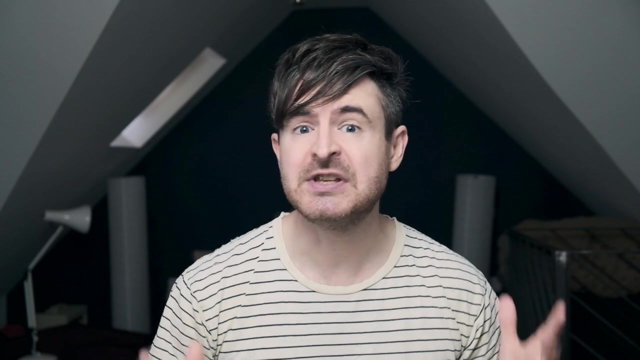 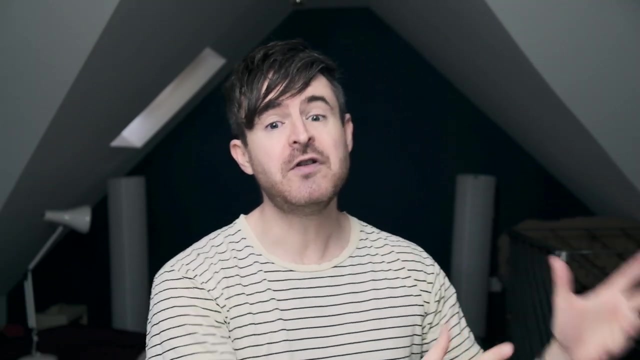 Hello everyone, Welcome to Attic Philosophy. We are doing a series of videos introducing the basic concepts of logic And this video is going to be on equivalence. Before you watch this one, make sure you've watched the previous video, which defines entailment. That's going to be. 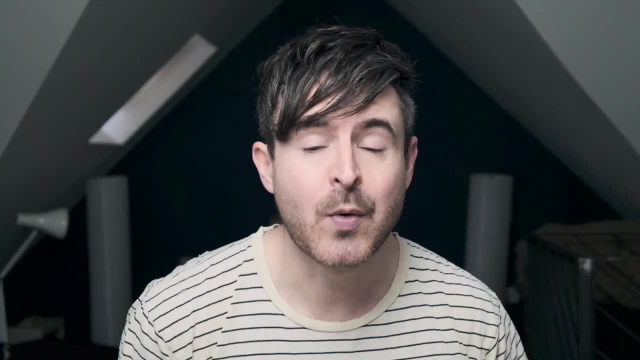 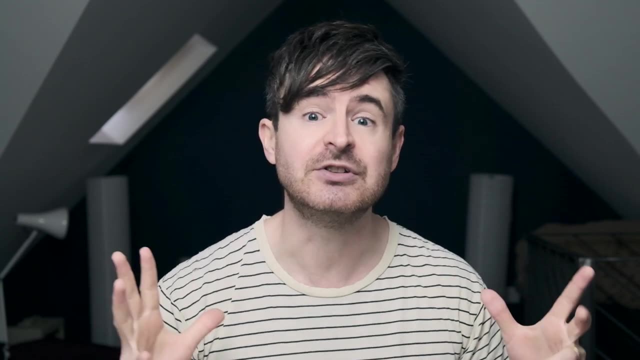 important to our understanding And we're going to be talking about the basic concepts of logic. We're going to look at equivalence in two parts. In this video, we're going to take a look at what equivalence is and how we check for it using truth tables, And then in the next video, we're going to 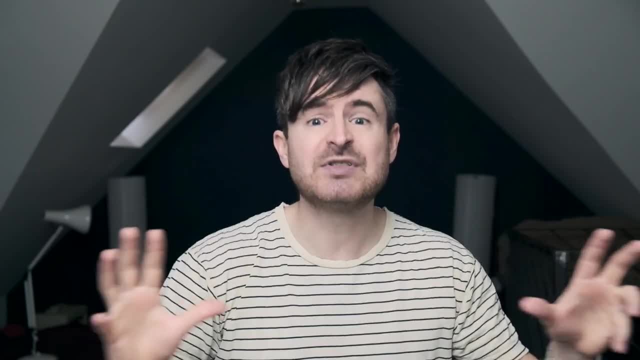 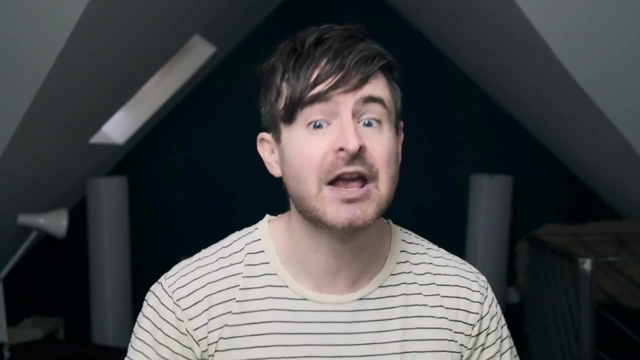 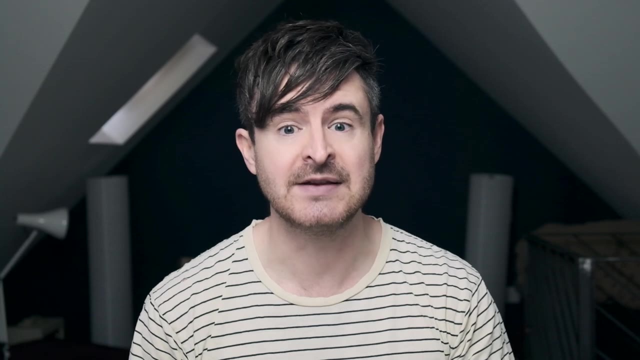 look at some equivalent schemes, That is, schemes that keep coming up, where we have two sentences which are guaranteed to be equivalent to one another, And then later on in the series we're going to see how to use those equivalent schemes to rewrite sentences in interesting ways. 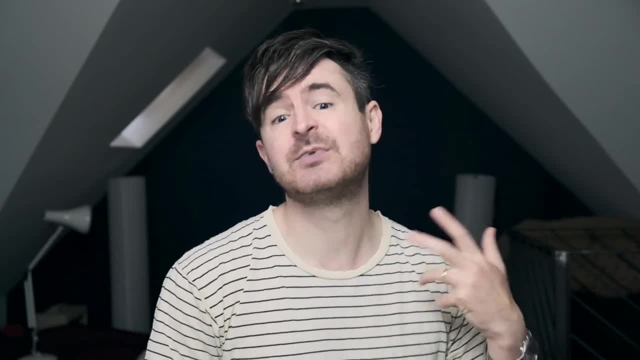 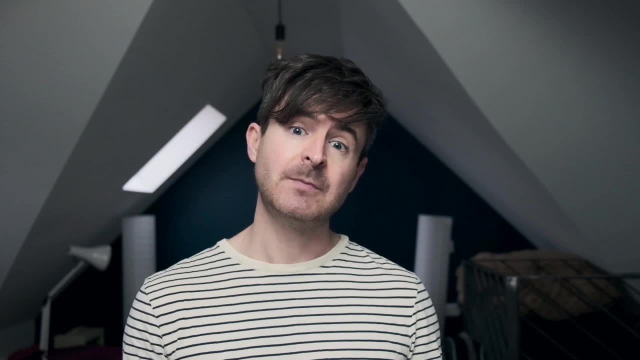 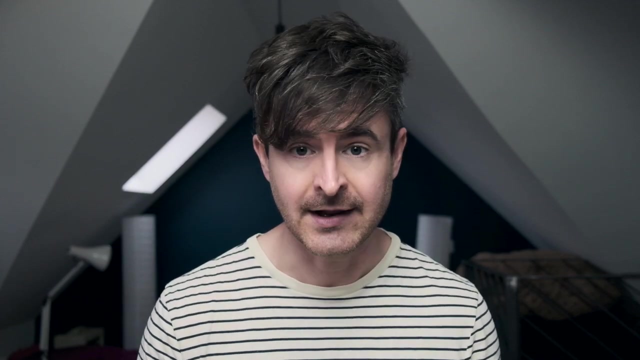 So if you're finding this series of videos useful, why not subscribe to the channel? hit the bell icon to get updates. Because we've already defined entailment, it's really easy for us to now define equivalence. It's simply two-way entailment. So when we have two sentences, A and B, 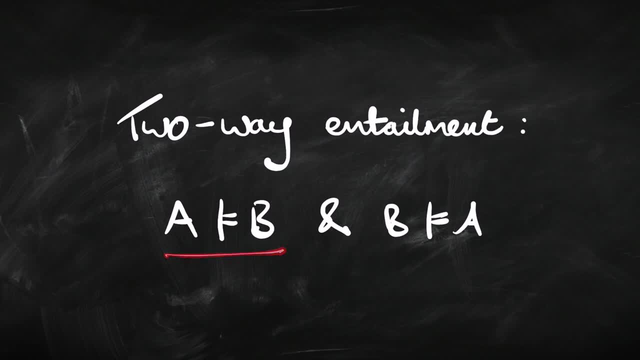 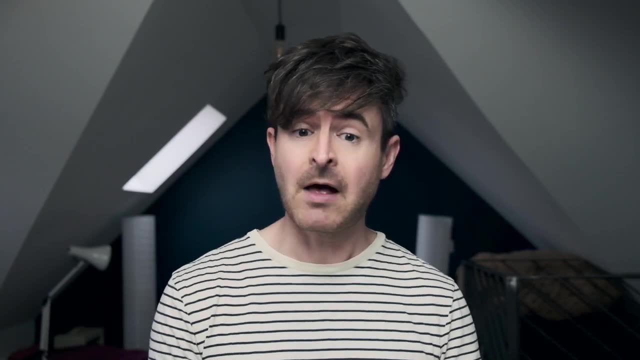 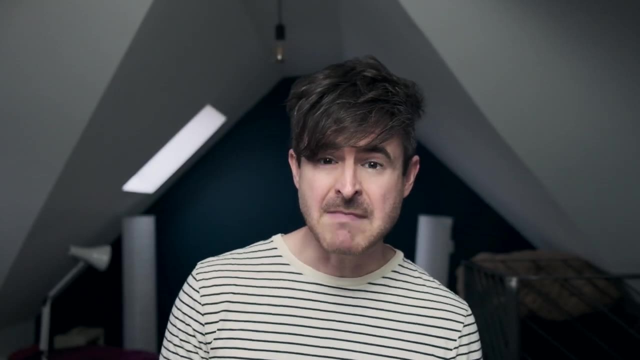 they are equivalent. just in case A entails B and also B entails A, It's good to have a symbol as a symbol for writing down that A and B are equivalent. Some logicians use this symbol- the three bars- You see that in maths quite a bit- to say that A and B are equivalent sentences. I'm not going to. 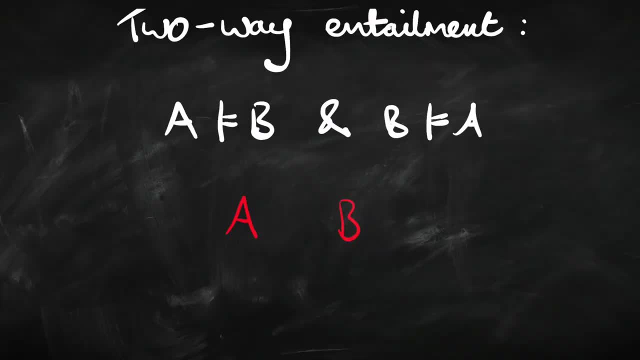 use that one. I'm going to use the symbol that we've already got. So we've got this one for saying that A entails B, and I'm going to write it backwards to say that A and B are equivalent. Okay, because it's like A entails B and B entails A. That's what we've got going. 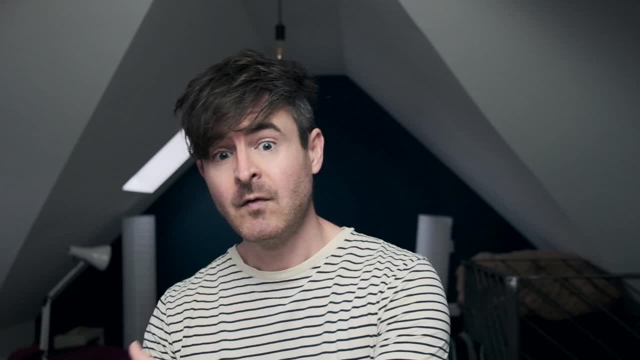 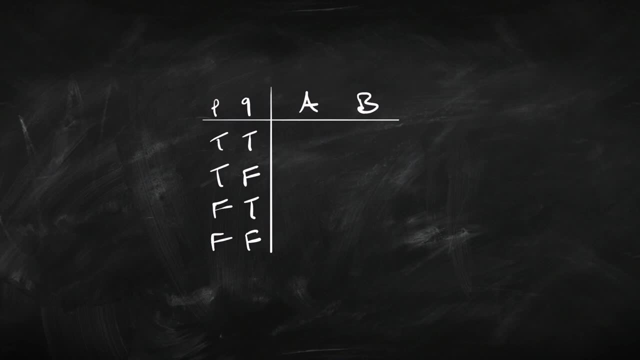 On here. So I'm using the entailment symbol forwards and backwards to denote equivalence. How would we use a truth table to work out whether A and B are equivalent? Well, we could just use the definition we've got and go the long way around and first of all see if A entails B. 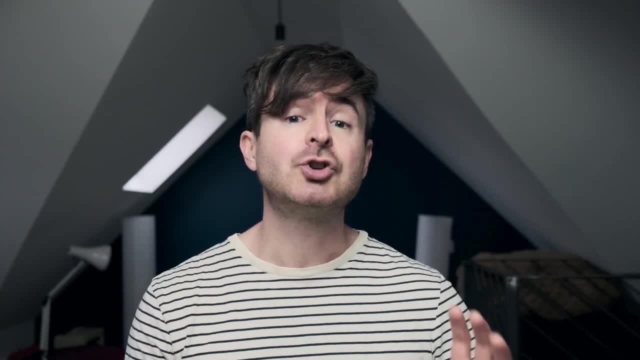 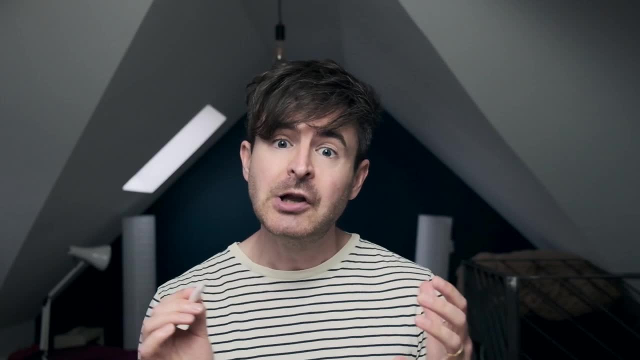 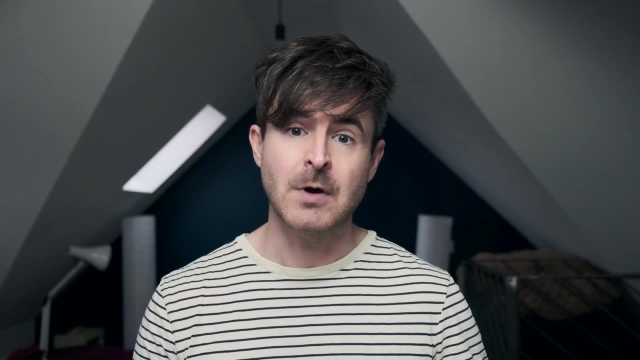 and then see if B entails A. But actually there's a much shorter way. All we need to do is check whether A and B have matching columns. Equivalence means that the truth table for A is exactly the same as the truth table for B. 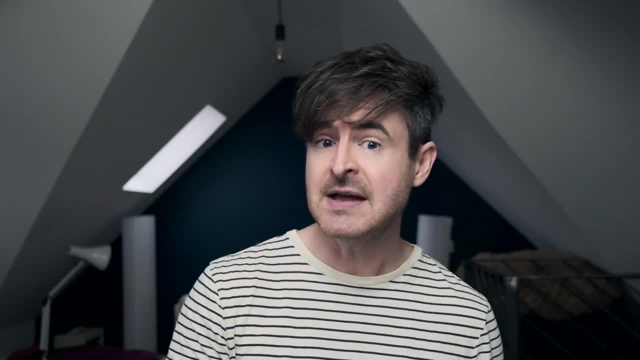 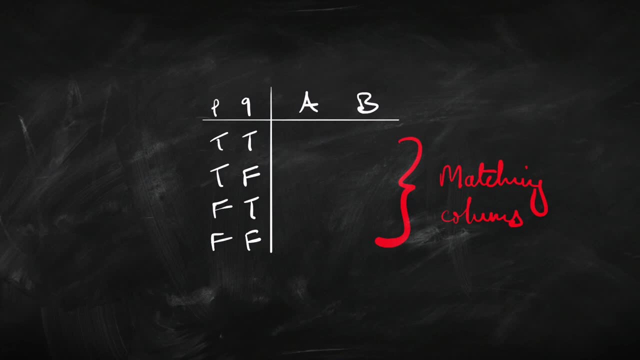 Okay, so in every line, if there's a T for A, there's got to be a T for B, And if there's an F for A, there's got to be an F for B. Matching columns for A and B. That's what logical equivalence. 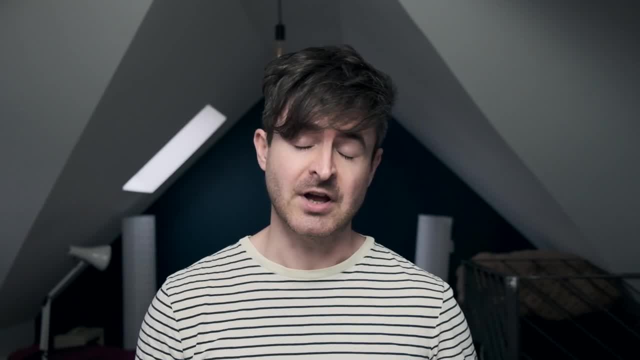 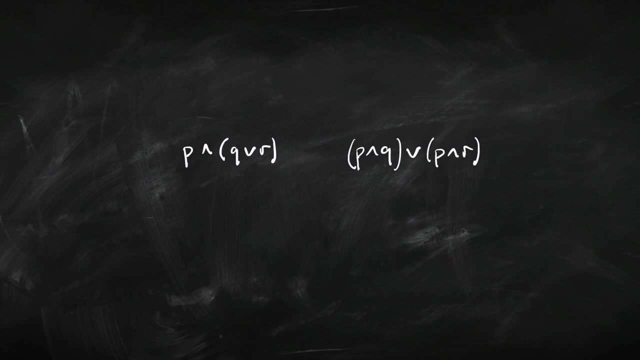 looks like in a truth table. Let's look at an example. Suppose we want to work out whether this sentence is logically equivalent to this sentence and we're going to do it using a truth table. How are we going to do that? First up, we're going to write both sentences down at the top. 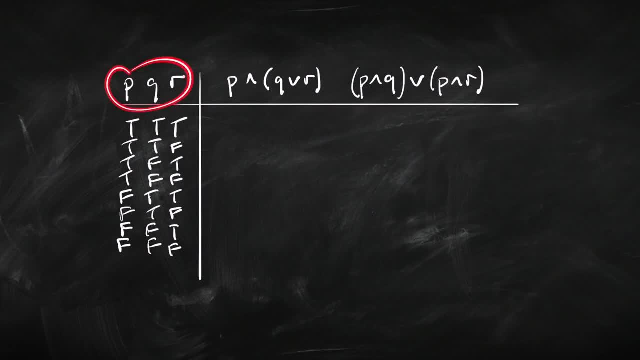 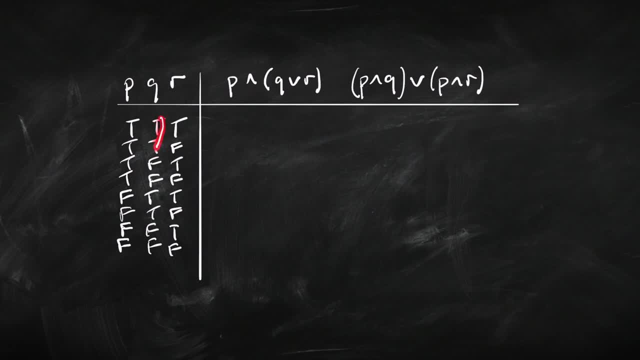 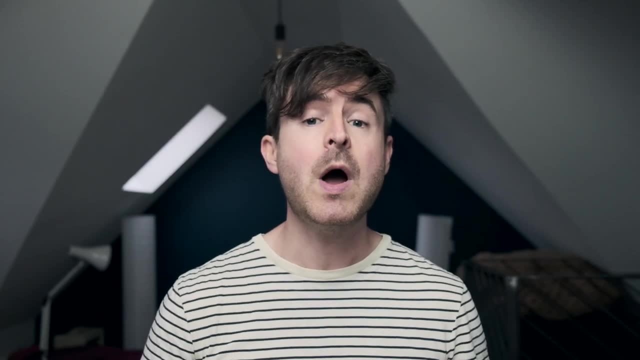 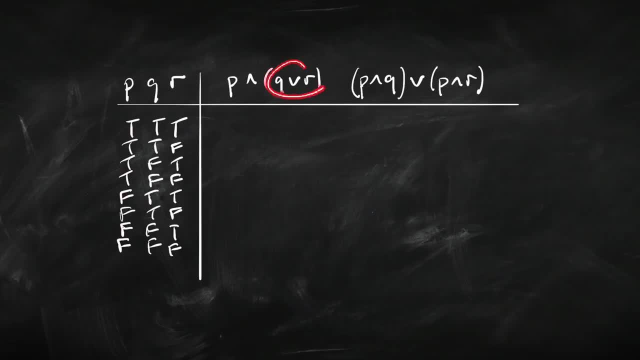 through these sentences sub-sentence by sub-sentence. Let's start here: Q or R, So there we're looking at whether there's a T in either the R column or the Q column, So that is going to look like this. Then we're looking at this whole sentence. That's an, and So we're looking. 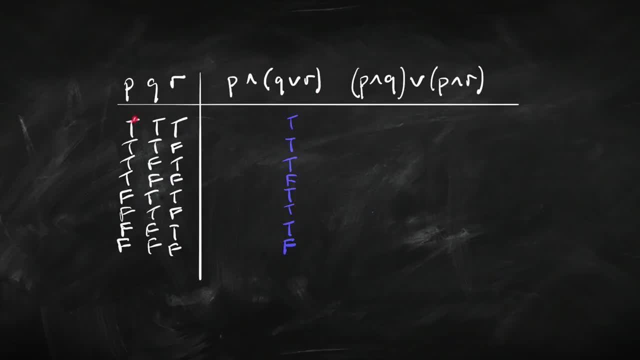 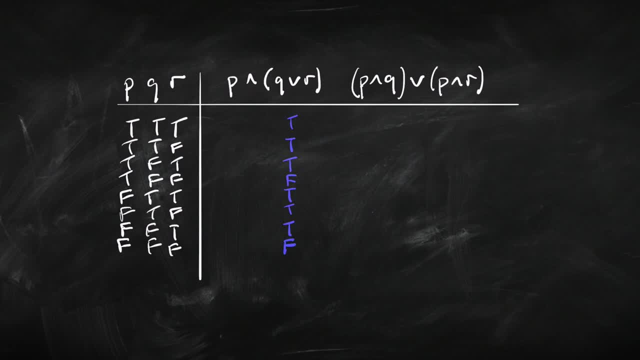 F, F. And since we're looking for a T in both columns, we kind of only need to look at the top four lines. So we look at the top four lines. Where have we got a T? It goes the first three lines. The rest of them are going to be Fs, like this. So three Ts and 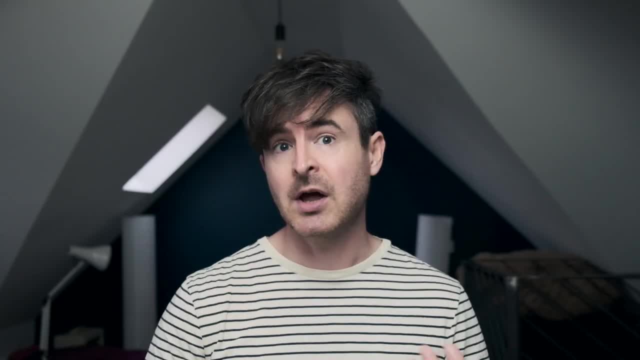 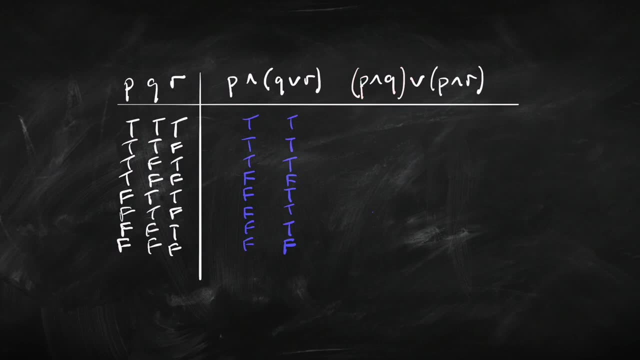 then five Fs. Now let's move over to the second sentence. Again we're going to go sub-sentence by sub-sentence. P and Q: Again we're looking for a T in both of those columns. And again we know there's only going to be a T in the first four lines And for Q it's just the. 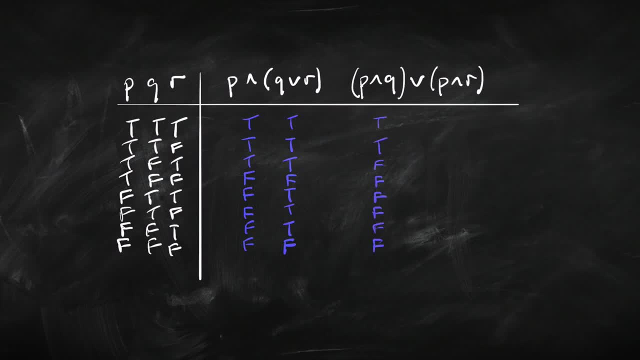 first two lines. So we're going to get two Ts, followed by six Fs, P and R. So we're looking for a T here and here And again. it's just those first four lines that we really care about, because those are the only Ts for the P, So we're going to get a T in the first. 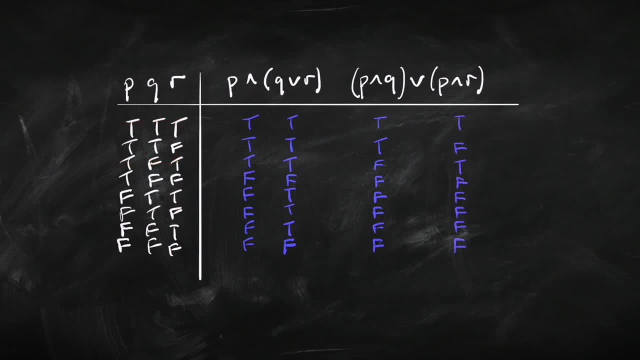 line and the third line. The rest of them are going to be Fs. Then let's look at this whole sentence. It's an OR. So we're looking at the two columns we've just done. Where do I have a T in one? 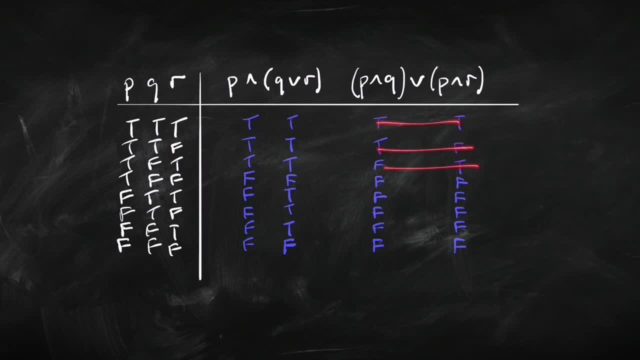 or other of them. So it's the first line, the second line, the third line and the rest of them are going to be Fs. So we've done an individual truth table for this sentence and an individual truth table for that sentence. Now we want to compare them, So we're going. 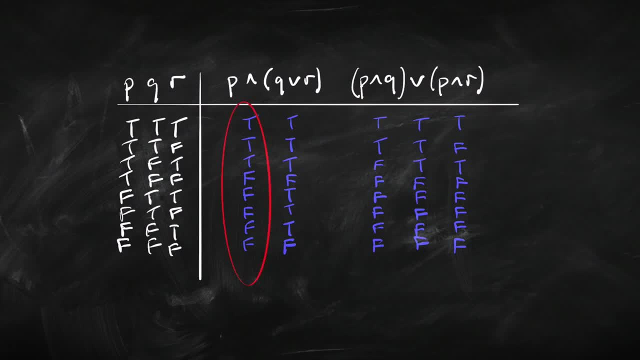 to be comparing this column and this column. So be really careful here. Remember the order in which you've written this sentence. So if you've written this sentence, you've worked through these different columns. We did this one first. That's like our working. 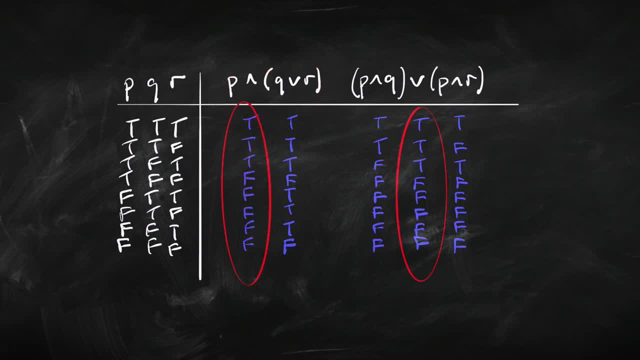 but here is our answer to this sentence. And similarly over on the right-hand side: this and this was our working, but this is our final answer for this sentence. So it's these two columns here that we want to be comparing, And then we just say, well, are they the same? 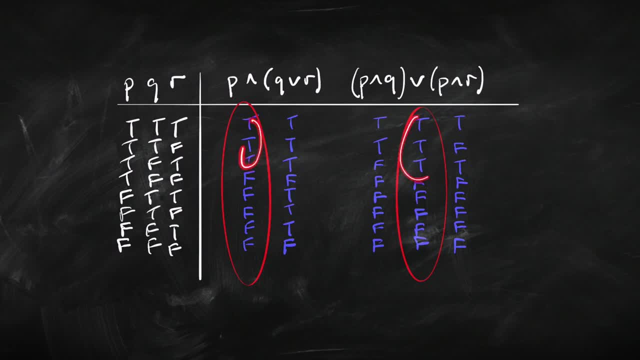 Check line by line. It goes T T T there, T T T there, and the rest of it's an F. It's the same column for both sentences, So those sentences are Equivalent. That is most of what we need to know about equivalence. We've looked at the 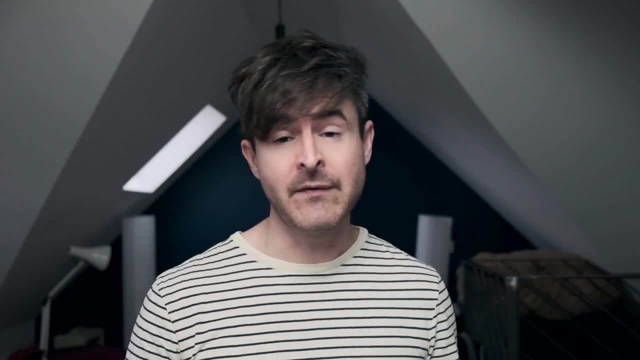 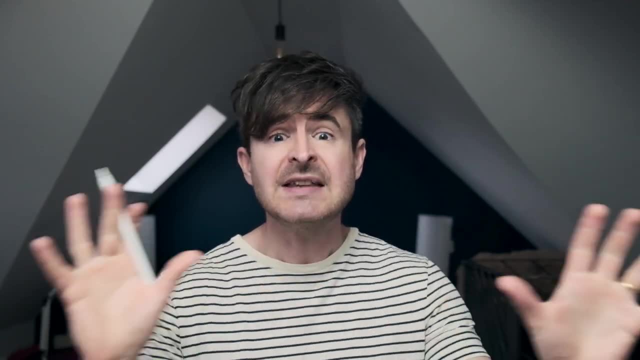 definition, two-way entailment, and we've looked at what equivalence looks like in a truth table, So we can always check for any two sentences whether they're equivalent or not. Okay, So that's the basics. That's most of what we need to know. However, there are some equivalences.